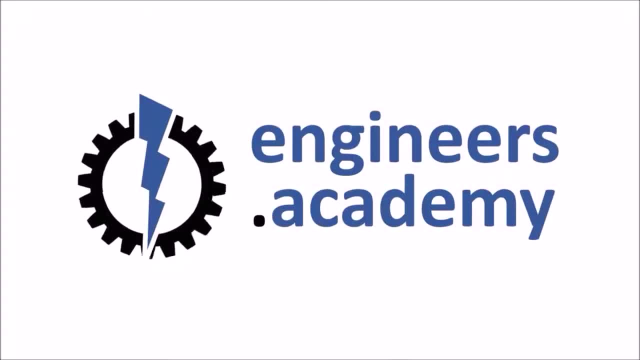 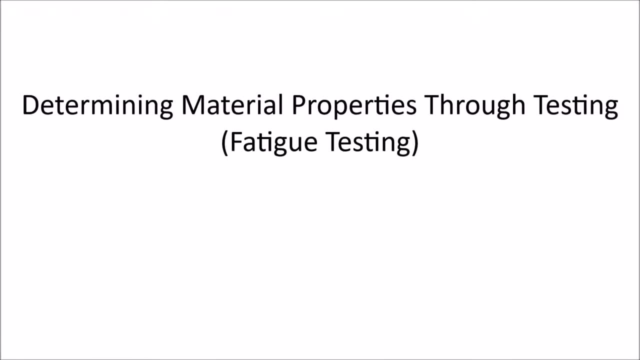 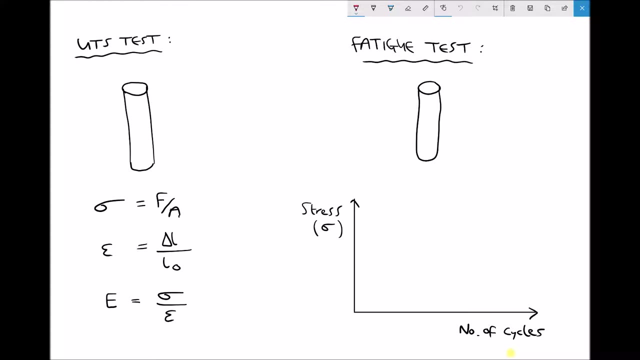 In this video we're going to discuss fatigue testing and we're going to make some comparisons with the UTS test that we've seen previously. Now we already know that in a UTS test, the type of load that we apply is a gradual load, So what we have is the bottom end of the test piece being 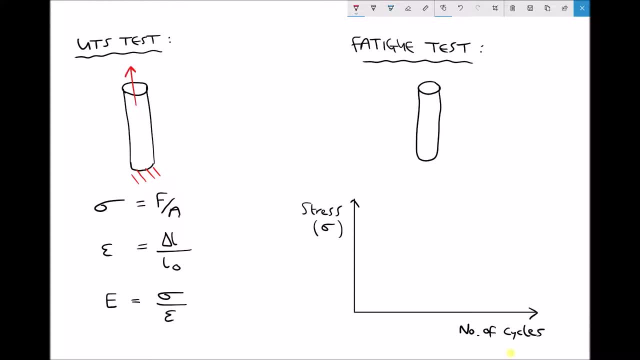 fixed and we're going to have a gradual increasing load being applied to the top of the test piece. So as the test progresses, the size of that force is going to increase, hence gradual loading. Now there's a couple of difference with fatigue testing, but first of all, the bottom of our test. 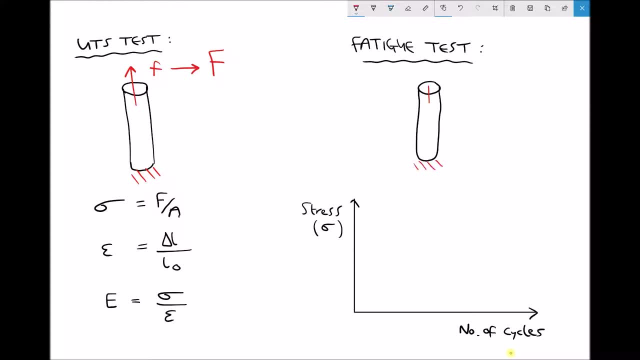 piece is still going to be fixed and we're still going to apply a force to the top of our test piece. The difference this time is that the force is going to be applied and then removed, and then applied and then removed. So what we have instead is cyclic loading. 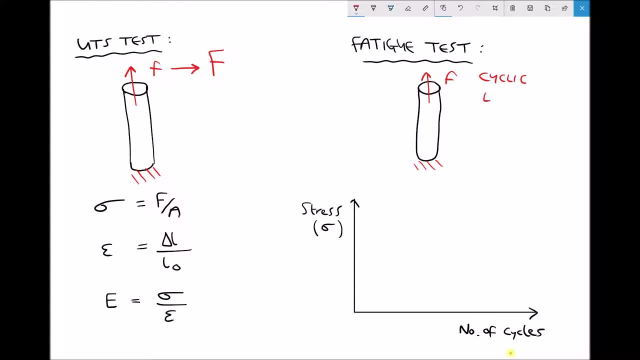 as opposed to the gradual loading that we see in a UTS test. Now, the ultimate tensile strength test machine can still be used for this test, but it has to be programmed to apply cyclic loading as opposed to gradual loading. So the way that this test would be conducted is the magnitude of the applied force would be. 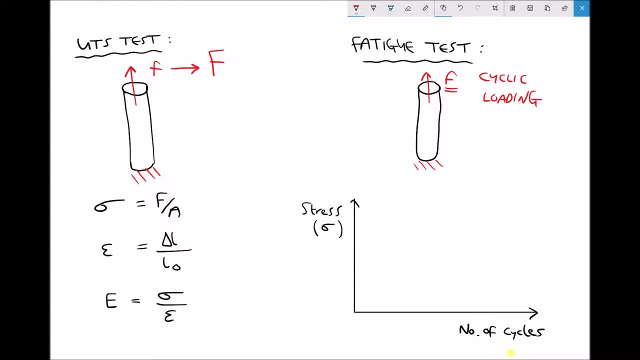 specified and the magnitude of the applied force would be the same for each cycle. From that force we could determine the amplitude of the cyclic stress, because we know that stress is force over area. So we would have a known applied stress and we would load an. 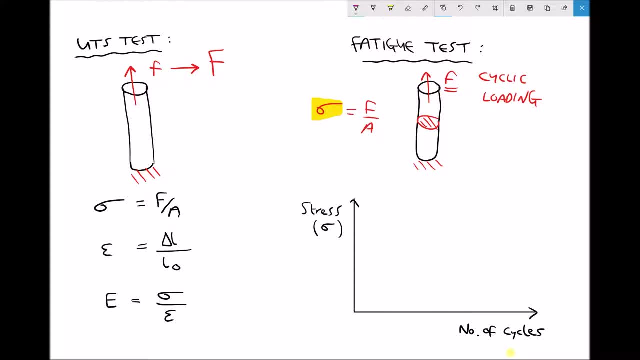 unload that sample until it failed. So let's say, for example, that the magnitude of the applied stress was 100 MPa And during that test we were able to do 10,000 cycles before the test piece failed Somewhere on this axis we would have a number of cycles of 10,000.